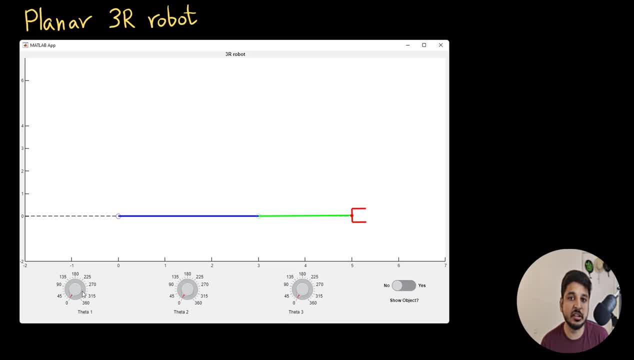 configuration is when all the robot parameters, which in this case are the three angles, theta1,, theta2 and theta3- are zero. And now I am going to increase theta1.. So you can see that the robot revolves as theta1 is increasing. So I am going to increase theta1.. So you can see that the robot 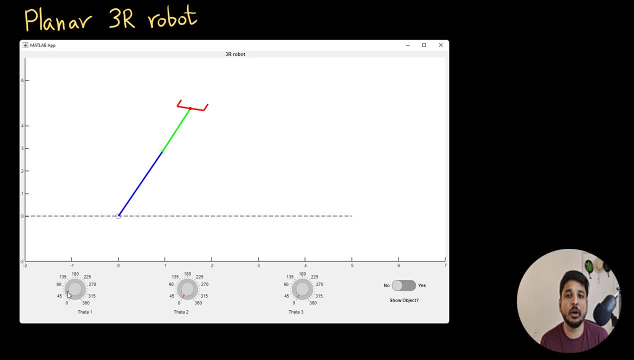 as theta1 is increased. Keep in mind that all the thetas are positive in the anti-clockwise direction. Now I am going to revolve theta2 and similarly theta3.. Now let me introduce an object into the space. So this is the object that the robot needs to pick up. 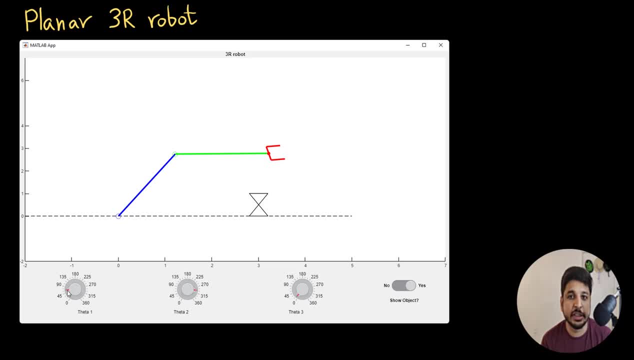 So the question is: in order to pick up this object, what should be the robot parameters? So how far should the motors rotate? That is, what should be the value of theta1, theta2 and theta3 to make the end effector come to such a position that it can grab the object Just by trying. 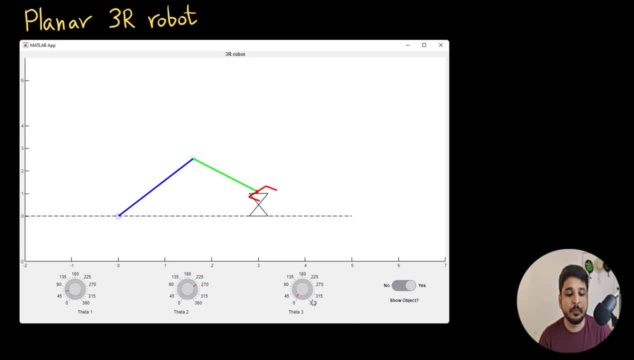 try an error. I can see that in this case it would be somewhere around 45 to 90 degrees for theta1,, somewhere around 225 to 270 degrees for theta2 and somewhere around 320 to 330 degrees for theta2.. Now let us do this numerically in a more exact manner. 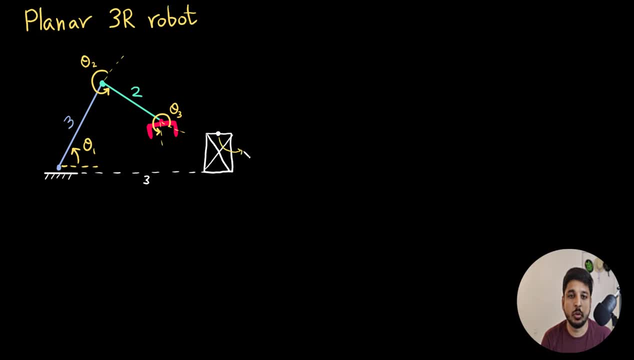 Now let me draw the object here. So the object is three units to the right and it has a height of one unit. So now the question is: what is the required location and orientation of the end effector so that it can pick the object? I know just by looking that the x coordinate must be 3,. 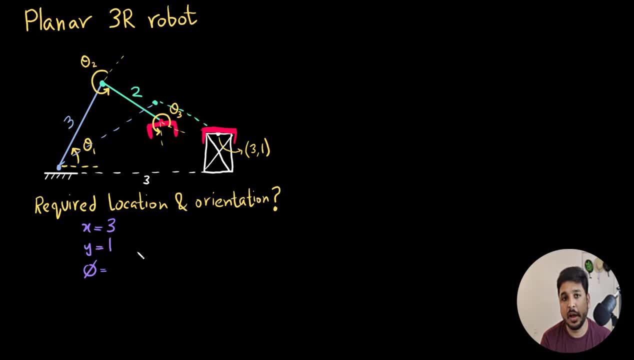 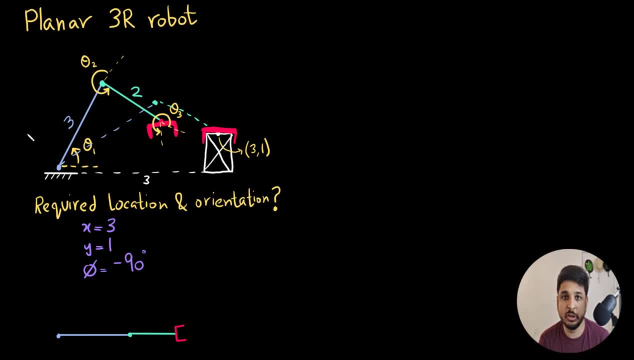 it is always a good idea to first draw the robot at the zero configuration, as drawn here. Mark out all the moving frames M1, M2 and M3, as well as the fixed frame. So compare this moving frame M3 with the location of the moving frame M1 and M3. 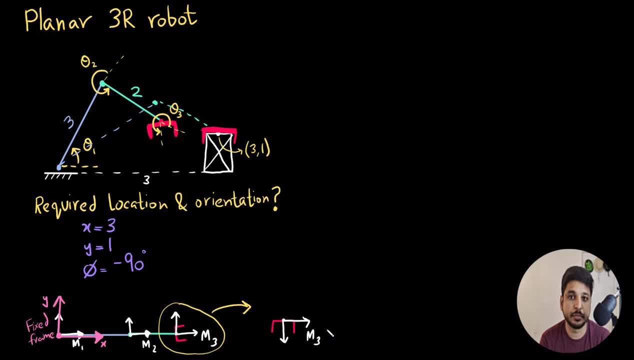 when the end factor is picking up the object and you can see that it has treated to 70 degrees in the anti-clockwise direction or 90 degrees in the clockwise direction, since, since anti-clockwise is positive, clockwise is negative, so it is minus 90 degrees. one thing to note is that 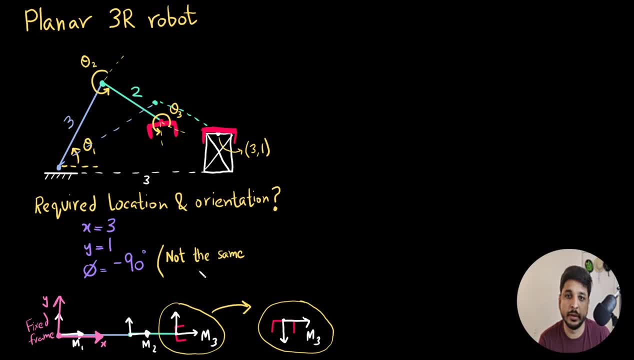 the orientation of the end factor is not theta 3.. now, in order to do inverse kinematics, what we first do is we write out the forward kinematics. if you don't know how to write forward kinematics or you just want to refresh your concept, i would highly recommend to check the video. 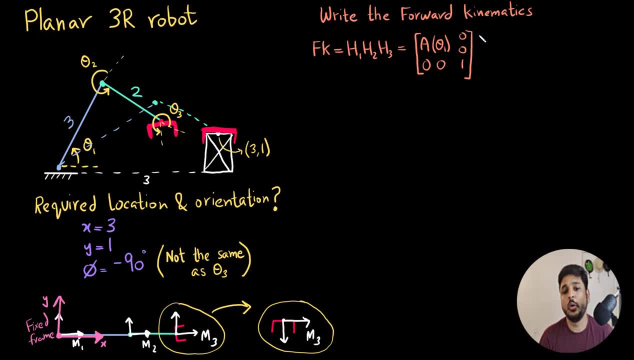 uh out. the link is in the description, so writing out the forward kinematics. it is comprised of three homogeneous transforms: h1, h2 and h3. the first homogeneous transform has zero displacement and a rotation matrix with the rotation angle theta one. the second homogeneous transform has 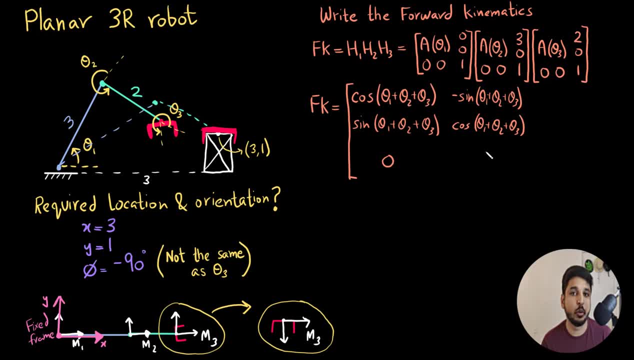 the displacement three units, and x, 0 and y and a rotation angle of theta 2, and the third has a rotation angle of theta 3 with 2 and 0 as the displacement. now, multiplying them out, i get this matrix right here. i know that this. 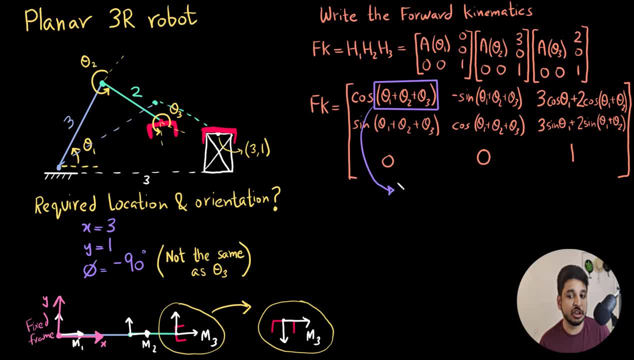 term, theta 1 plus theta 2 plus theta 3, is the orientation of the end effector, and these two terms gives me the location of the end effector, which is the x and y coordinates. so what i do now is i just expand the location with the required orientation at the location and i get these following three: 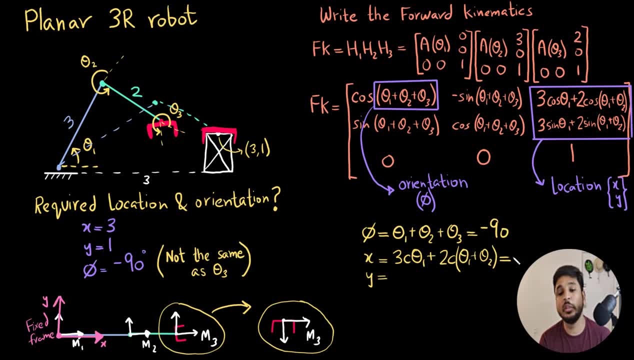 equations, and here i have three equations with three unknowns, so i know that these can be solved. now you have a number of ways to solve this. you can either solve it in a software, which i would highly recommend, but it's always good to know how to solve it, uh, using a pen and paper. so let me 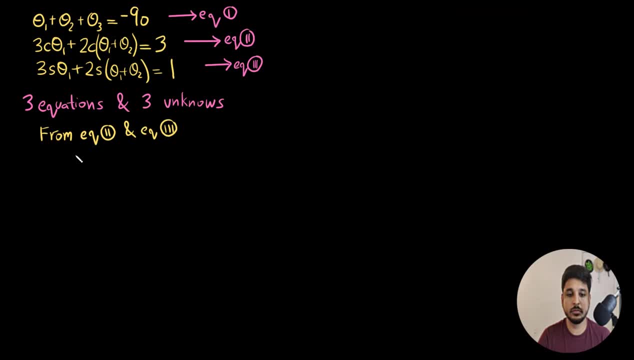 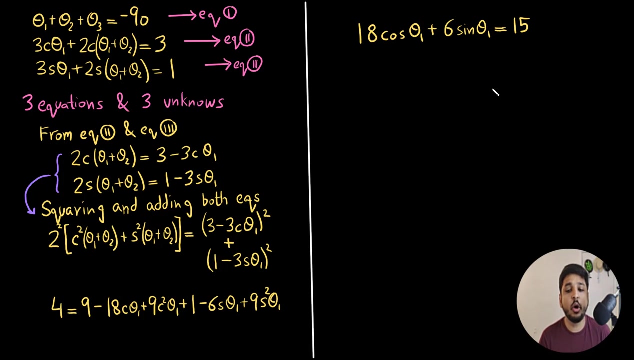 show you how. feel free to skip if you want to. so i'm going to go ahead and do this, and i'm going to do this very quickly. i'm just manipulating with the equations, squaring the equations up, adding the equations up, and i get to this point where i get 18 cosine of theta 1 plus 6 sine of theta 1 equals to 15.. now, in order, 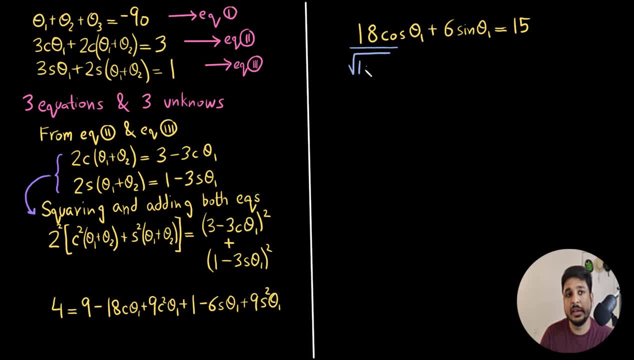 to solve this, there is a very nice technique that you can use. what this technique is is that you just divide all of the terms by the square root of the sum of the squares of the cosine and the sine terms. what i mean is that you divide them by the square root of 18 square plus 6 square. what we do is we then substitute: 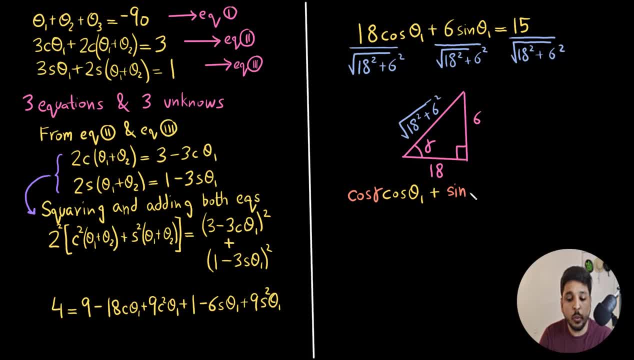 in place of this, the cosine of a new angle, which is gamma, and the sine of gamma. and we know from this right angle triangle that gamma is known and gamma can be found out. found out, so, solving further, i can see that i have a equation in theta which has gamma and plus, minus, cosine, inverse of something. 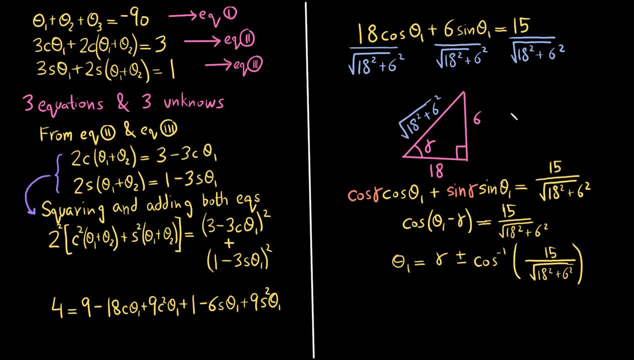 and i can always figure out gamma as being just the 10 inverse of 6 over 18.. so i get this equation. notice that this equation has a plus minus cosine inverse term, which means that i am going to get two values of theta. so that is what i get. so i get two values of theta 1.. i call them theta 1 a and theta. 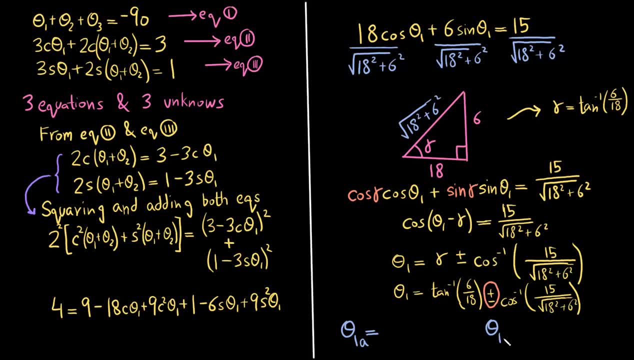 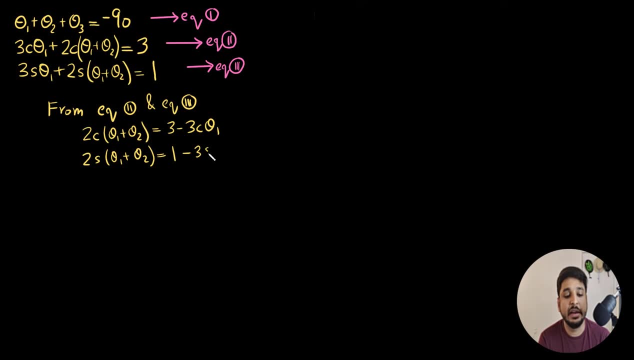 1 b. they represent two different solutions. that is something to keep in mind. the first solution has theta 2 degrees. the next has theta 1 as 19.3 degrees. now, fast forwarding again. i am just manipulating these equations and i am finding out theta two values again. i am going to get two. 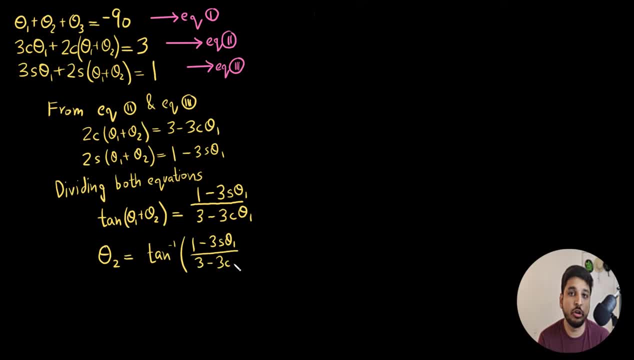 different values: theta 2a and theta 2b. theta 2a corresponds to the solution the first solution, which is theta 1a, and theta 2b corresponds to theta 1b. similarly, using the third equation, i get two values of theta 3. 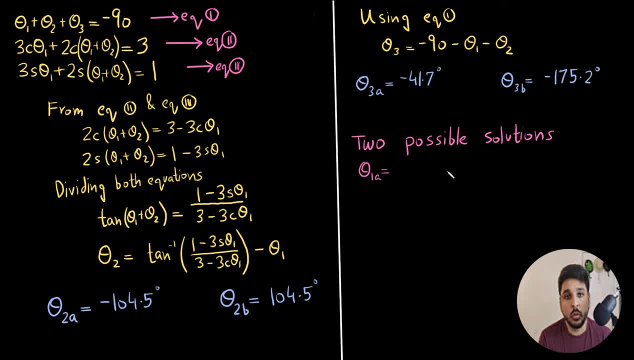 which are a and theta 3 b. so at the end i get two possible solutions. so i get two possible solutions. the first solution has theta 1 as 56.2 degrees, theta 2 as minus 104.5 degrees and theta 3 as